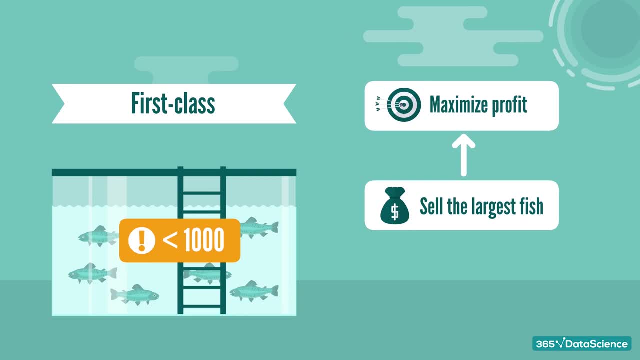 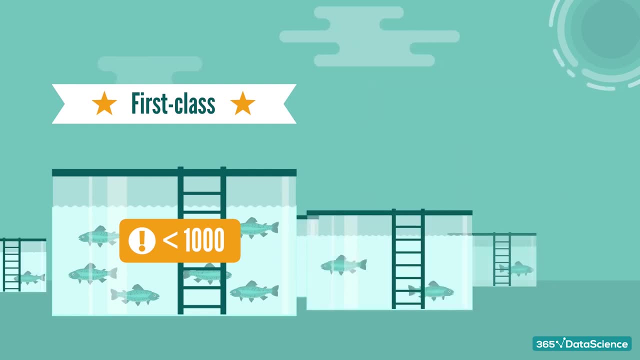 All things considered, selling the first-class fish as large as possible would be your best strategy to increase profit. Therefore, you need to maximize the length of each fish in every single tank. Easy to say, but how can you do that? How long is it going to take? 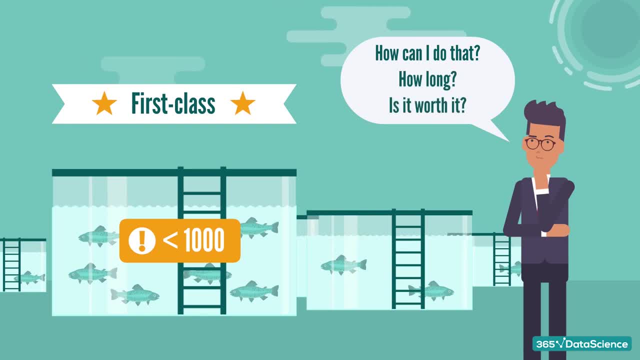 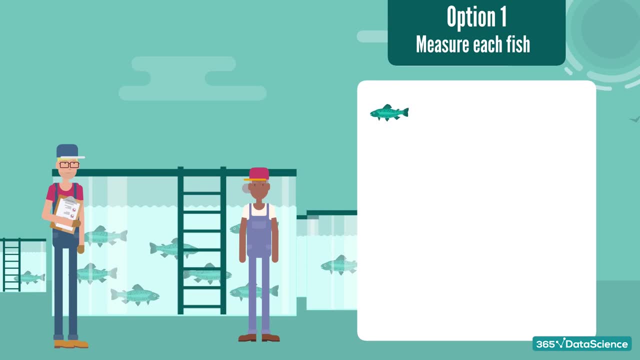 Is the effort worth the time you will lose while in competition with other fish farms? Let's think about it for a second. One option is to try to measure each fish separately, but there are 1,000 fish in each tank and more than 20 tanks stocked with first-class fish. 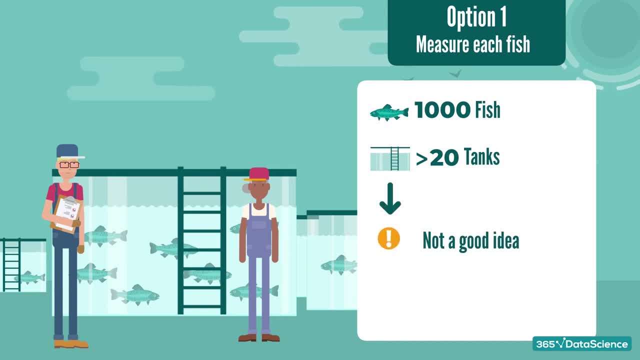 So manually measuring each fish doesn't sound like a good idea. It will simply take too long. You and your employees will be stuck measuring fish from dawn till dusk, which is highly inefficient. What's more, if you can quickly find out the average size of your fish, 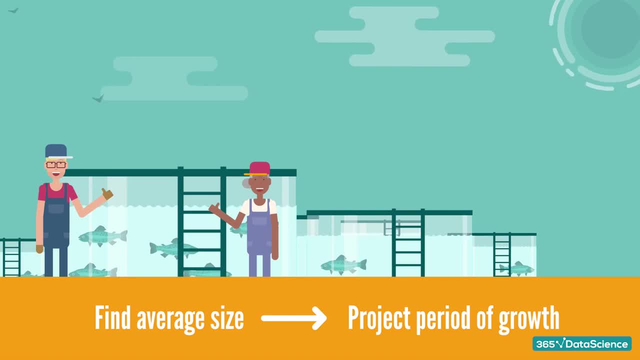 you can project how long it will take for each tank to grow the necessary size. This will allow you to plan key resources such as staff and fish food supplies. Finally, having an edge in the business depends on your ability to stay competitive and agile. 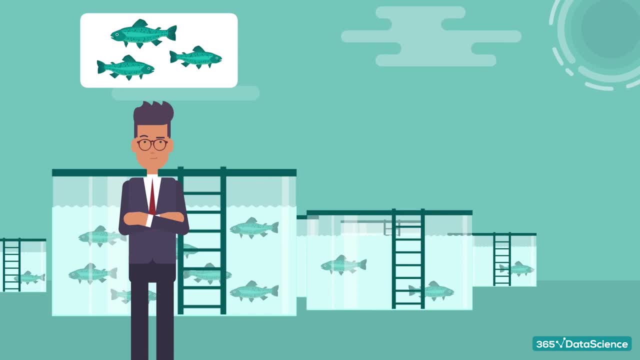 Knowing what kind of sales volumes you can produce daily helps you to be prepared when a customer calls to purchase a certain number of tanks due a particular date, And this is where you can truly benefit from some maths knowledge. to optimize the process More precisely, you can use the central literature. 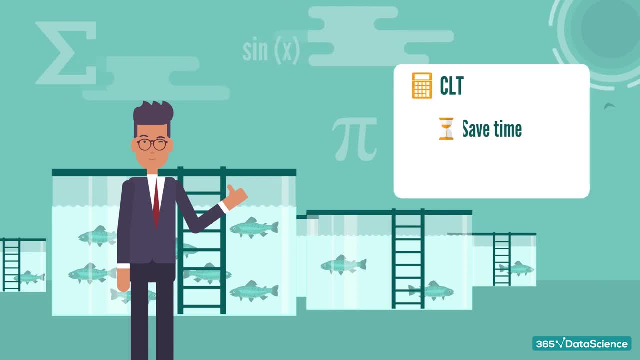 more precisely. you can use the central literature, as it is a fundamental part of the Central Limit Theorem. Plus, it will help you tremendously with time saving And, what's more, you will also maximize your profit at the same time. 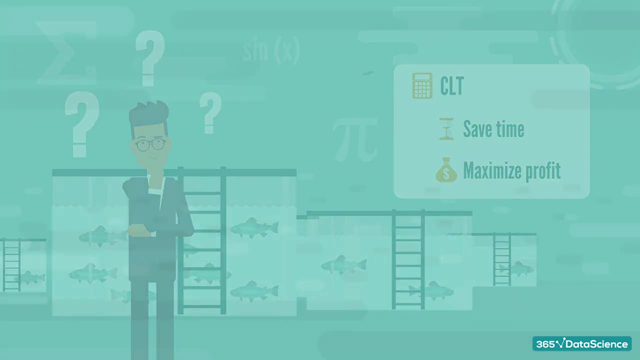 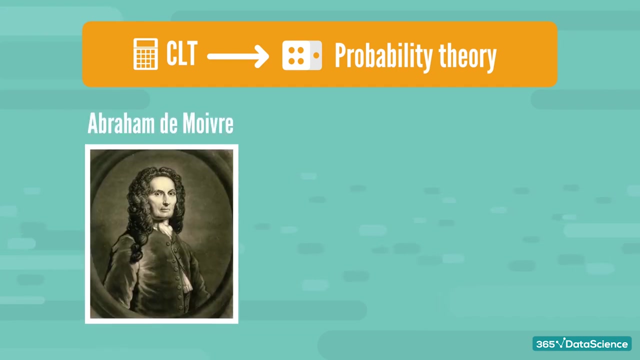 So what is the Central Limit Theorem and how does it work? The Central Limit Theorem is a theorem in probability theory whose first version was proposed by the French mathematician Abraham de Moivre in 1733.. Moivre published an article where he used a normal distribution. 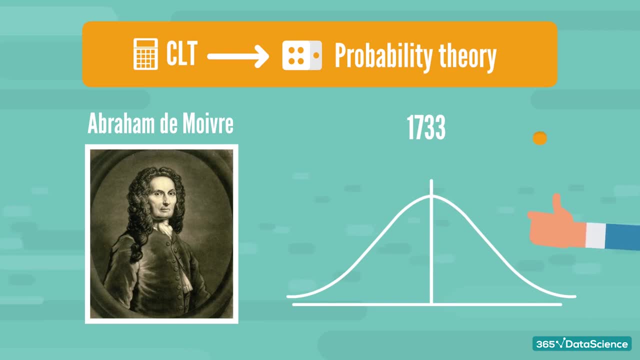 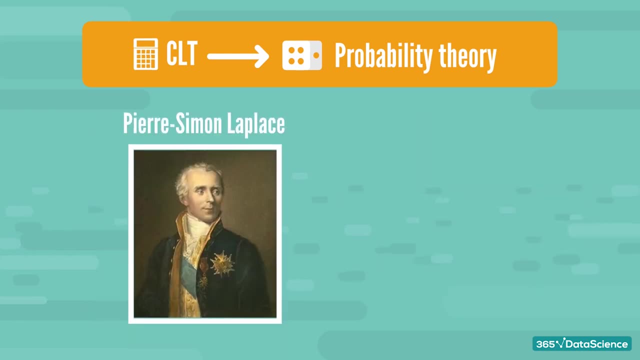 to approximate the distribution of the number of heads resulting from many tosses of a fair coin. The finding was nearly forgotten until the French mathematician Pierre-Simon Laplace expanded it in his monumental work in the 19th century. Over the years, numerous versions of it have been discovered and proven by other mathematicians. 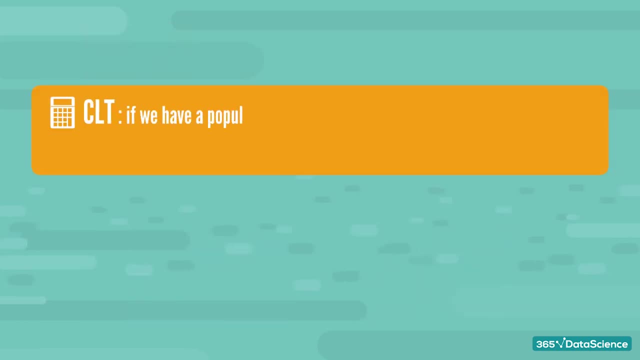 In its base form, the central limit theorem states that if we have a population and we take sufficiently large random samples from it, then the sample means will be approximately normally distributed. We call the average of each sample a sample mean, In case you're wondering what a sample mean is. 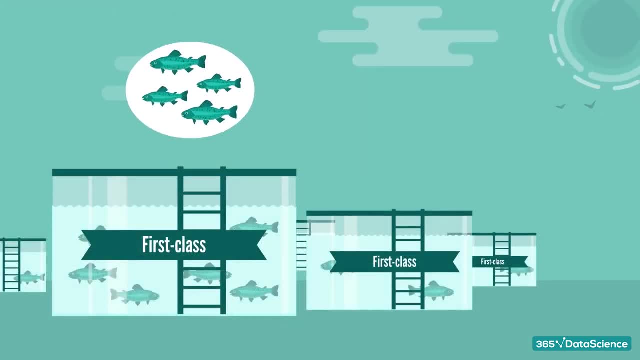 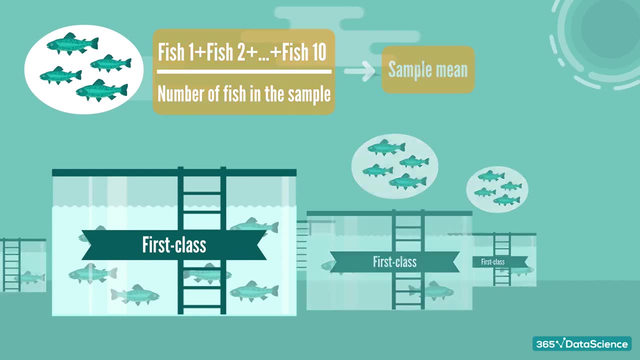 let's go back to our fish example and see: If you simply take groups of fish from each first-class reservoir and record the average size in each group, that would be the so-called sample means. In fact, that's exactly how the central limit theorem can be applied to improve our fish measuring dilemma. 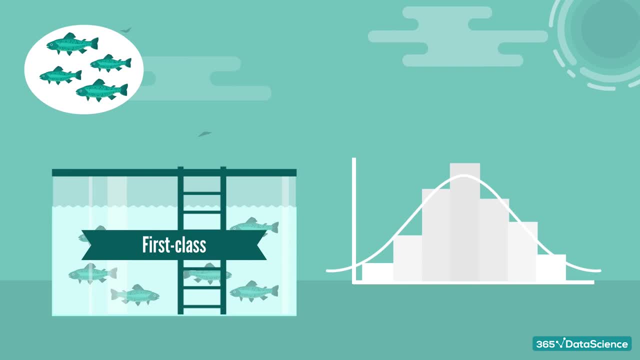 Let's see it in practice. It's a rule of thumb that the minimum sample size to apply the CLT on is 30. That's why we start with a sample size of 30. That means each group of fish you select from your 1,000 first-class fish reservoir. 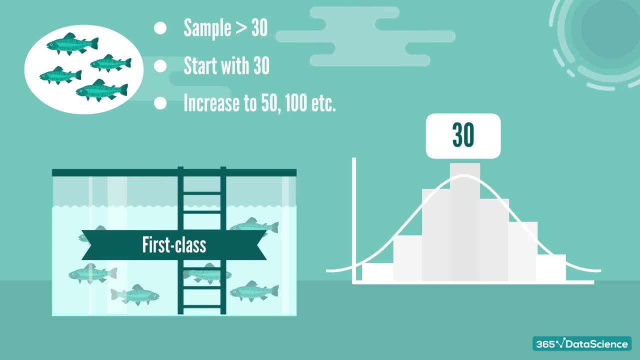 will consistently consist of 30 fish. Then you'll increase the sample size to 50,, 100, etc. And each time you record the sample mean. the idea is to gradually increase the sample size, because the bigger the sample, the better the theorem applies. 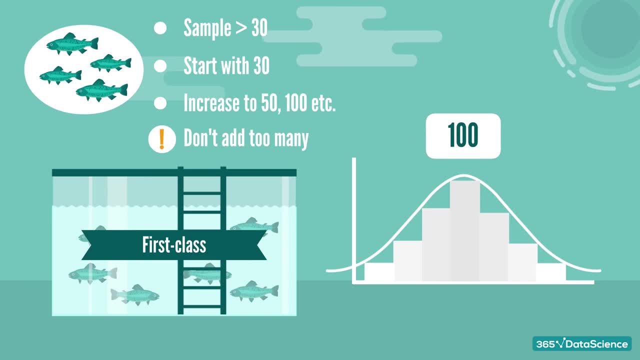 However, you must not try with too many values for sample sizes, because you want to be able to act as quickly as possible for each first-class tank. So there are two possible outcomes. The size of fish in the respective pool is the maximized one: 50 cm. 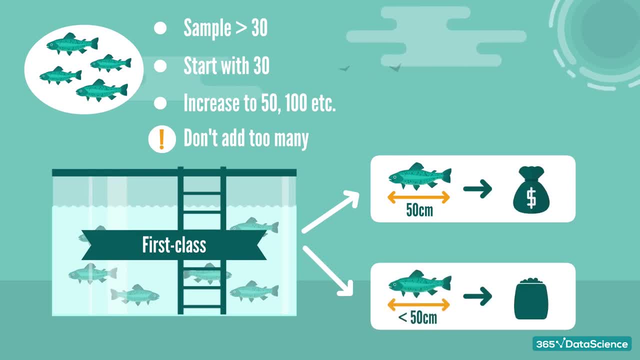 which means you can sell the whole tank or you must keep feeding them and take measurements at a future date. Then you do this for each first-class reservoir After recording and plotting. the sample means you can see. the plot fits under the bell-shaped curve. 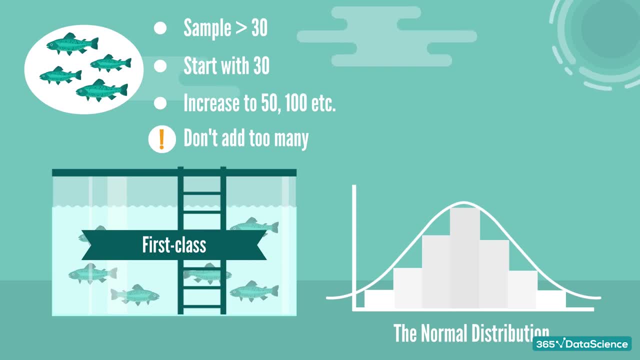 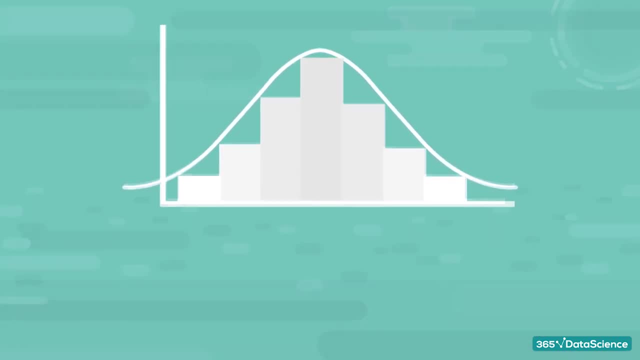 illustrating the normal distribution. Therefore, going forward, you are in a position to perform a statistical analysis using the properties of this distribution. From the normal distribution graph you see that the middle is denoted by mu, the mean of sample means, which divides the area into two equal and symmetric halves. 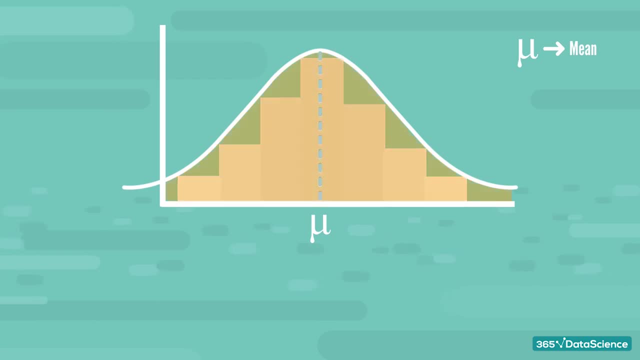 Moreover, the area under the curve, which is this area here, is equal to one. The first key observation is that approximately two-thirds of the collected means are one standard deviation away from the mean of sample means, and approximately all of the data lies within two standard deviations away from it.